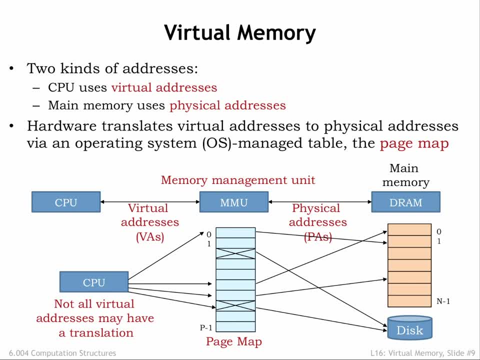 haven't yet been loaded into main memory. This would indicate that the contents of the requested virtual address haven't yet been loaded into main memory. So the MMU would signal a memory management exception to the CPU, which could assign a location in physical memory and perform. 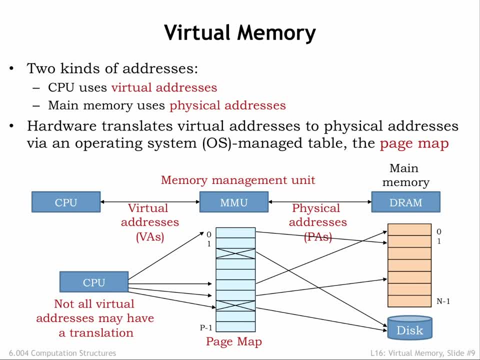 the required I-O operation to initialize that location from secondary storage. The MMU table gives the system a lot of control over how physical memory is accessed by the program running on the CPU. For example, we could arrange to run multiple programs in quick succession. 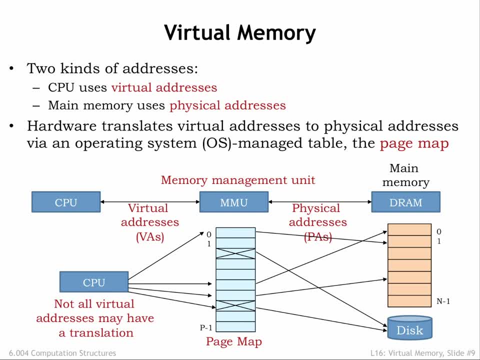 by changing the page map. when we change programs, Main memory locations accessible to one program could be made inaccessible to another program by proper management of their respective page maps, And we could use MMU exceptions to load program contents into main memory on-demand instead of having to load the entire program before execution starts. 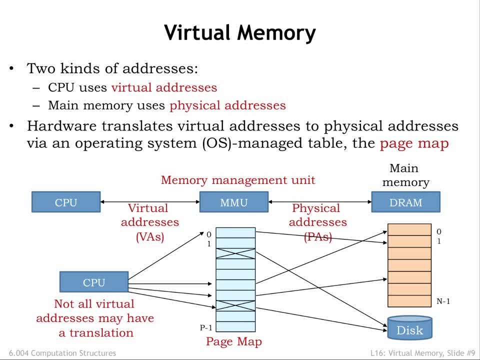 In fact, we only need to ensure the current working setup of a program is actually resident in main memory. Locations not currently being used could live in secondary storage until needed. In this lecture and next we'll see how the MMU plays a central role. 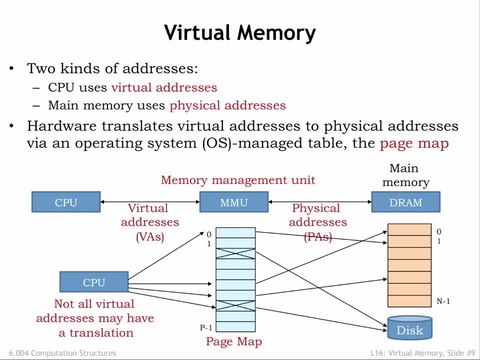 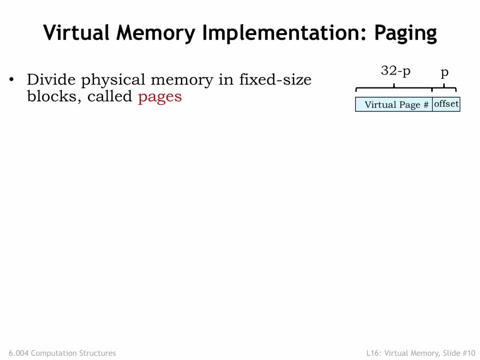 in the design of a modern time-sharing computer system. Of course we'd need an impossibly large table to separately map each virtual address to a physical address. So instead we divide both the virtual and physical address spaces into fixed-sized blocks called pages. Page-size blocks are usually divided into two individual sections. Page-size blocks are: 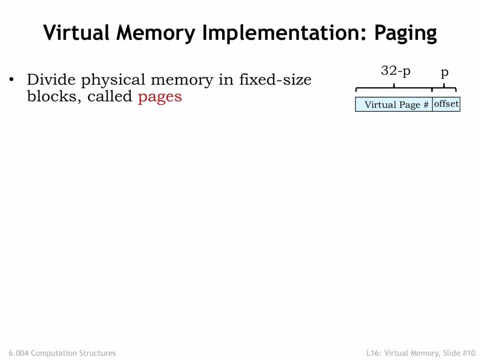 Adresses are always a power of 2 bytes, say 2 to the p bytes. so p is the number of address bits needed to select a particular location on the page. We'll use the low-order p bits of the virtual or physical address as the page offset. 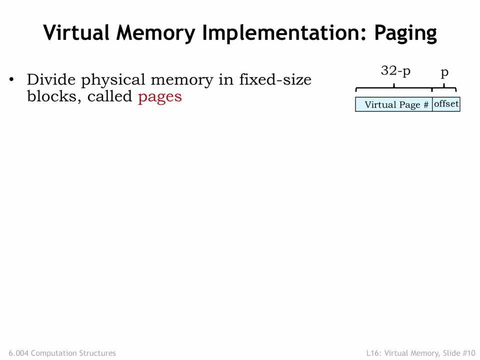 The remaining address bits tell us which page is being accessed and are called the page number. A typical page size is 4 to 16 KB, which corresponds to p equal 12 and p equal 14, respectively. Suppose p equals 12.. 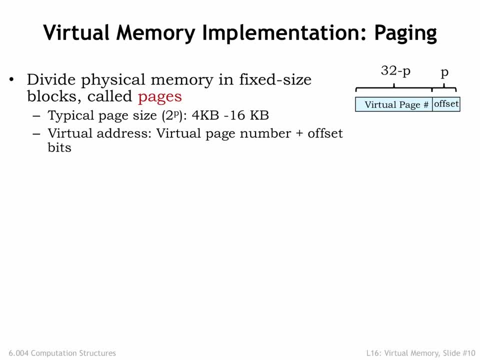 If the CPU produces a 32-bit virtual address, the low-order 12 bits of the virtual address are the page offset and the high-order 20 bits are the virtual page number. Similarly, the low-order p bits of the physical address are the page offset and the remaining 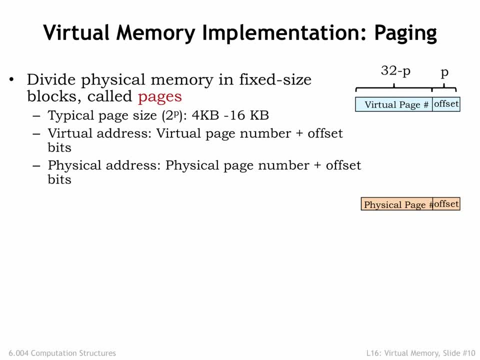 physical address bits are the physical page number. The key idea is that the MMU will manage pages, not individual locations. We'll move entire pages from secondary storage into main memory By the principle of locality. if a program accesses one location on a page, we expect. 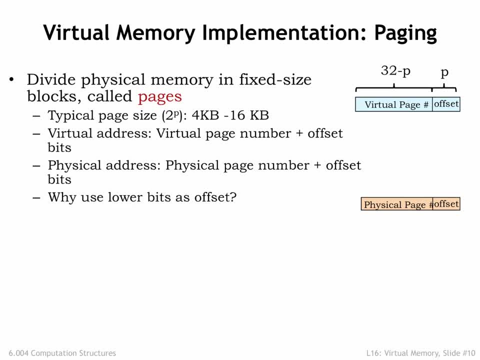 it will soon access other nearby locations. By choosing the page offset from the low-order address bits, we'll ensure that nearby locations live on the same page, unless, of course, we're near one end of the page or the other, So pages naturally capture the notion of locality. 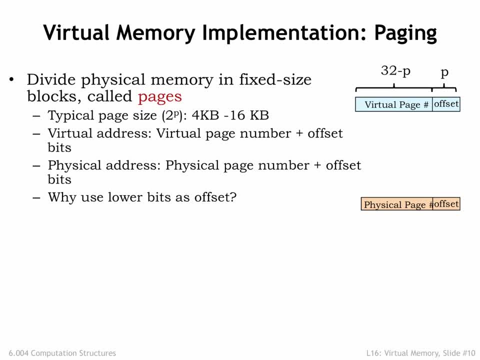 And since pages are large, they can be moved from the secondary storage to the main memory If the number of pages is large. by dealing with pages when accessing secondary storage, we'll take advantage that reading or writing many locations is only slightly more time-consuming. 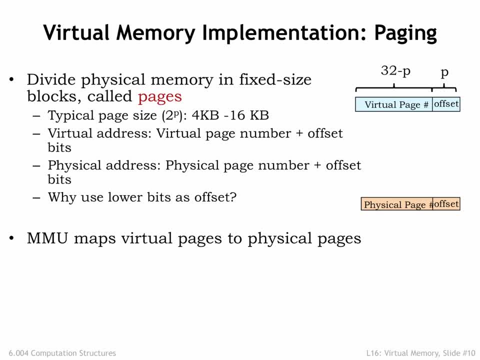 than accessing the first location. The MMU will map virtual page numbers to physical page numbers. It does this by using the virtual page number as an index into the page table. Each entry in the page table indicates if the page is resident in main memory and if 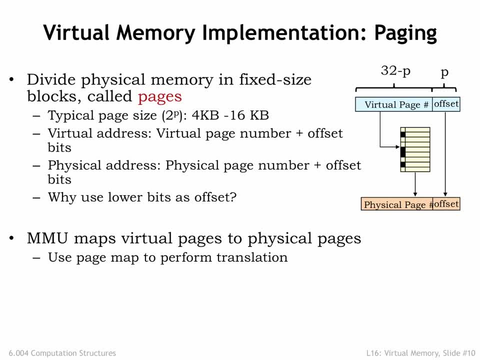 it is provides a new location. The mmu, which will form the address for the page, provides the appropriate physical page number. The physical page number is combined with a page offset to form the physical address for main memory. If the requested virtual page is not resident in main memory, the mmu signals a memory management. 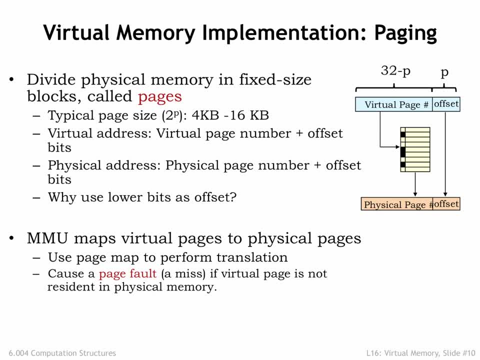 exception to the CPU so it can load the appropriate page from secondary storage and set up the appropriate mapping in the mmu. We'll do that next time. Bye, bye, called paging or sometimes demand paging, since movements of pages to and from secondary storage is determined by the demands of the program. 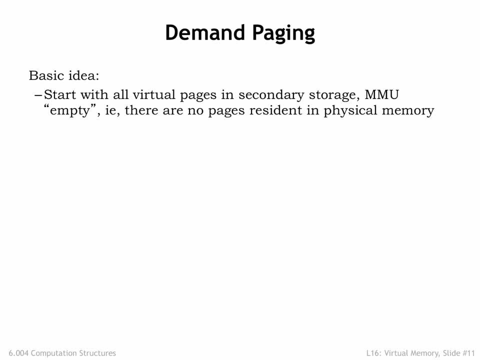 So here's the plan. Initially, all the virtual pages for a program reside in secondary storage and the MMU is empty. In other words, there are no pages resident in physical memory. The CPU starts running the program and each virtual address it generates, either for an 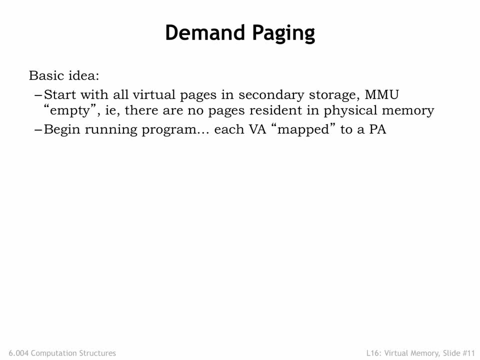 instruction, fetch or data access is passed to the MMU to be mapped to a physical address in main memory. If the virtual address is resident in physical memory, the main memory hardware can complete the access. If the virtual address is not resident in physical memory, the MMU signals a page fault. 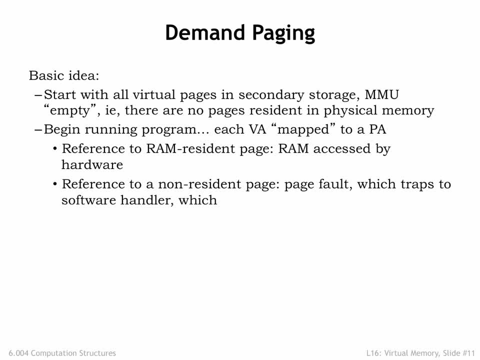 exception forcing the CPU to switch execution to special code called the page fault handler. The handler allocates a physical page to hold the requested virtual page. The handler then loads the virtual page from secondary storage into main memory. It then adjusts the page map entry for the requested virtual page to show that it is 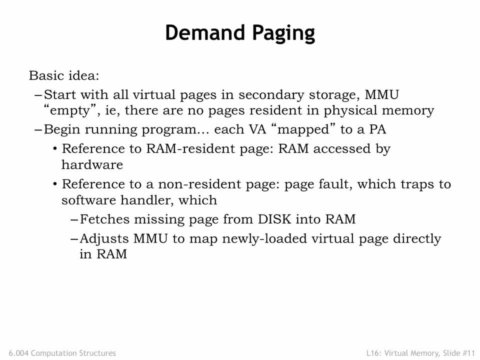 now resident and to indicate the physical page number for the newly allocated and initialized physical page. When trying to allocate a physical page, the handler may discover that all physical pages are currently in use. In this case, it chooses an existing page to replace. 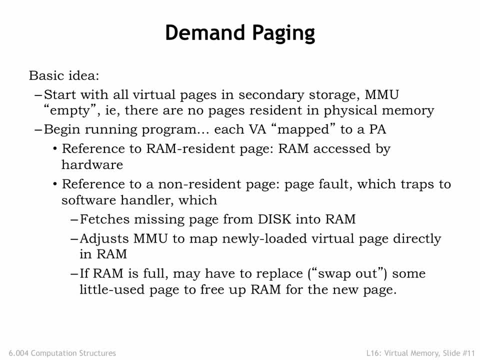 For example, a resident virtual page that hasn't been recently accessed. It swaps the contents of the chosen virtual page out to secondary storage and updates the page map entry for the replaced virtual page to indicate that it is no longer resident. Now there's a free physical page to reuse to hold the contents of the virtual page that. 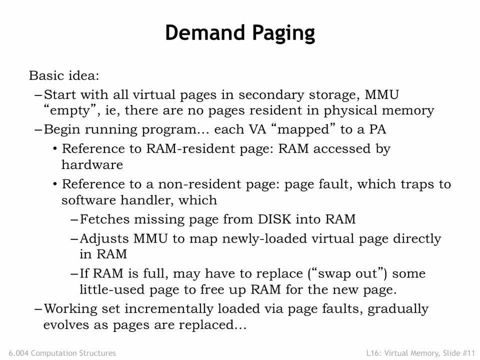 was missing. The working set of a program, ie the set of pages the program is currently accessing, is loaded into the VM. It is loaded into main memory through a series of page faults. After a flurry of page faults, when the program starts running, the working set changes slowly. 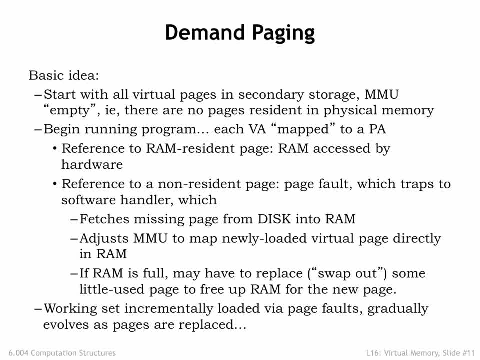 so the frequency of page faults drops dramatically, perhaps close to zero, if the program is small and well-behaved. It is possible to write programs that consistently generate page faults, a phenomenon called thrashing. Given the long access times of secondary storage, a program that's thrashing runs very. 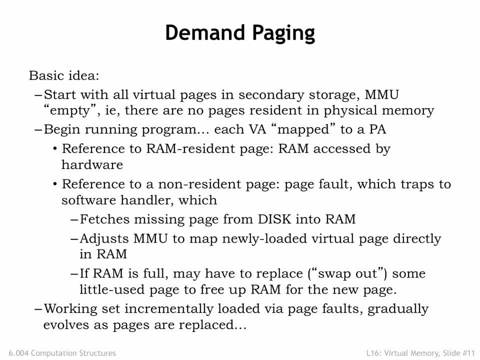 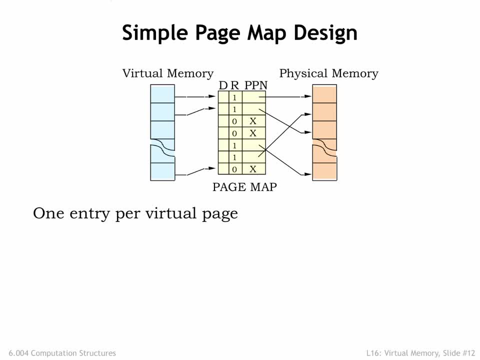 slowly, usually so slowly that the users give up and rewrite the program to behave more sensibly. The design of the page map is straightforward. There's one entry in the page map for each virtual page. For example, if the CPU generates a 32-bit virtual address and the page size is 212 bytes, 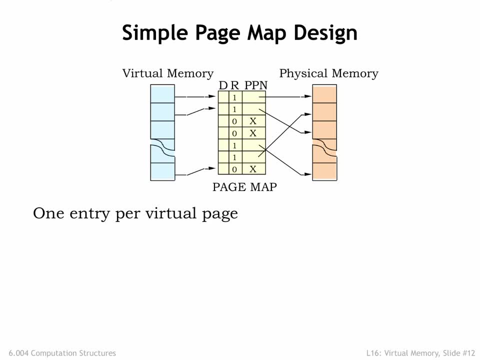 the virtual page number has 32 minus 12, or 20 bits and the page table will have 2 to the 20th entries. Each entry in the page table contains a resident bit r, which is set to 1 when the virtual 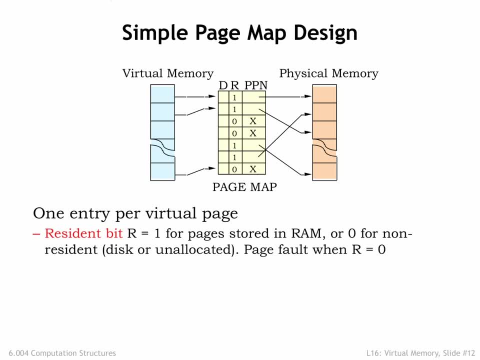 page is resident in physical memory. If r is 0, an access to that virtual page will cause a page fault. If r is 1, the entry also contains the physical page number indicating where to find the virtual page in main memory. 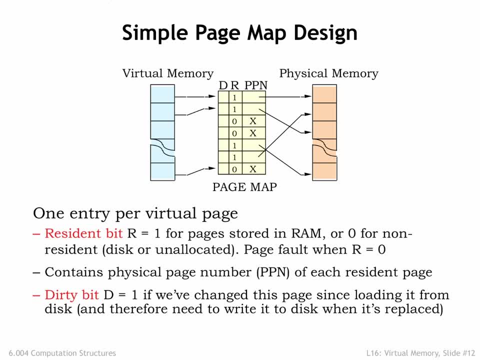 There's one additional state bit called the dirty bit d. when a page has just been loaded from secondary storage, it's clean, ie the contents of physical memory match the contents of the page in secondary storage. So the d-bit is set to 0. 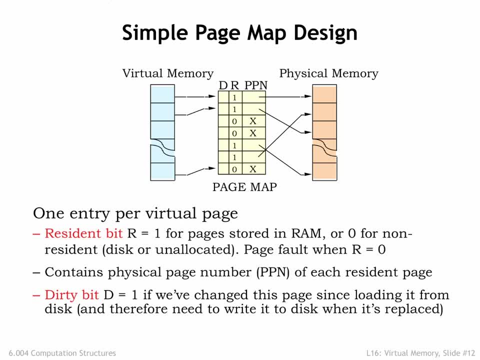 If subsequently the CPU stores into a location on the page, the d-bit for the page is set to 1, indicating the page is dirty, ie the contents of memory now differ from the contents of secondary storage. If a dirty page is ever chosen for a replacement, it's clean. 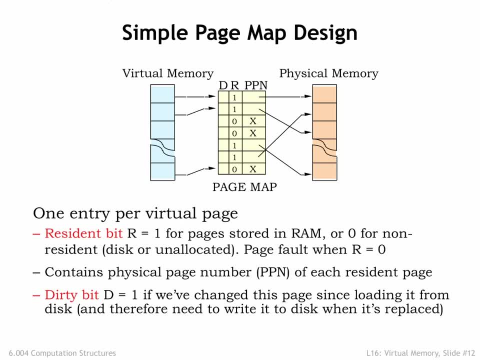 Its contents must be written to secondary storage in order to save the changes before the page gets reused. Some MMUs have additional state bits in each page, table entry, For example, there could be a read-only bit which, when set, would generate an exception. 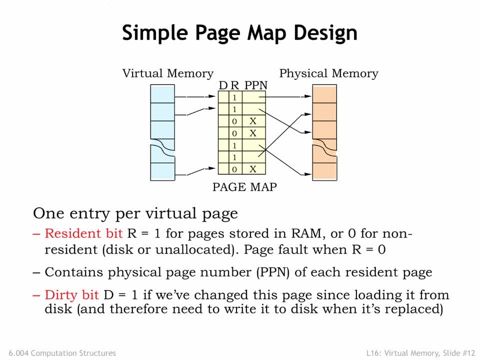 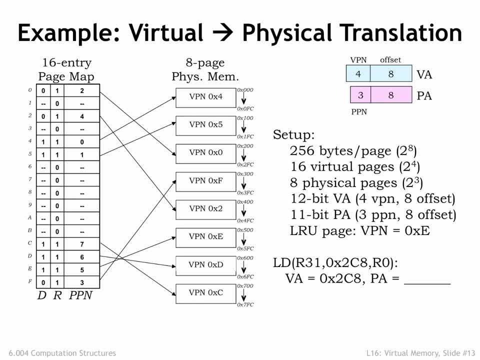 The MMU in action. To make things simple, assume that the virtual address is 12 bits, consisting of an 8-bit page offset and a 4-bit virtual page number. So there are 2⁴ or 16 virtual pages. 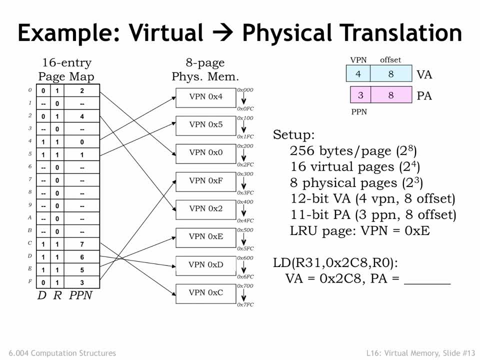 The physical address is 11 bits divided into the same 8-bit page offset and a 3-bit physical page number, so there are 2⁴ or 8 physical pages. On the left we see a diagram showing the contents of the 16-entry page map, ie an entry for each virtual page.